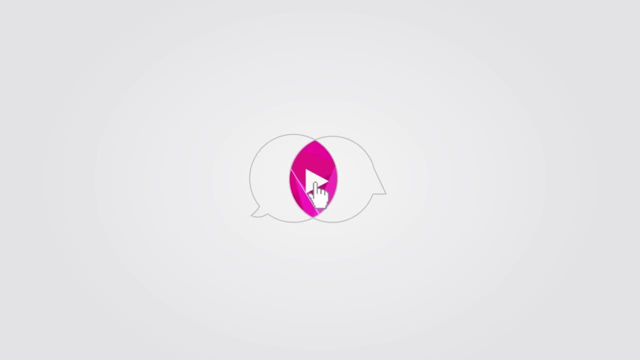 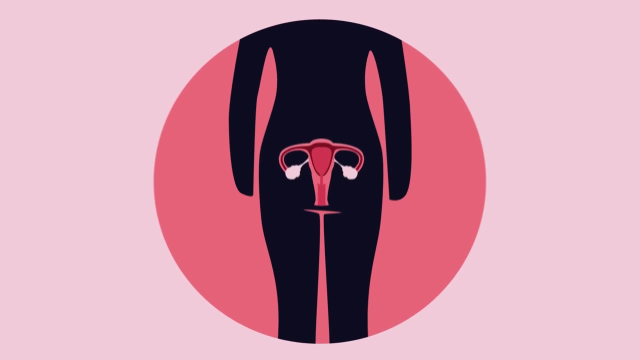 Men are from Mars, women are from Venus, and though we may share a planet and many other similarities, our bodies function in some majorly different ways. In this video, we'll take a look at some of those differences unique to women. Women between the ages of 12 and 50 years old undergo a monthly cycle in which their 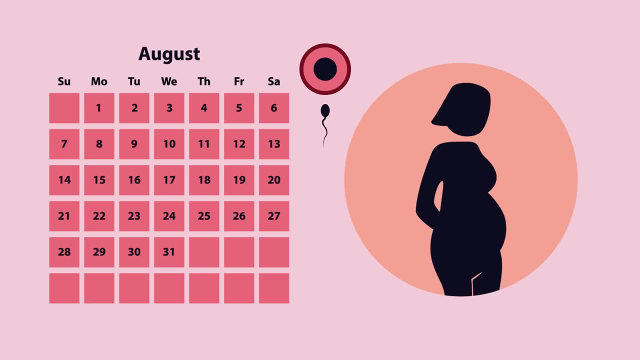 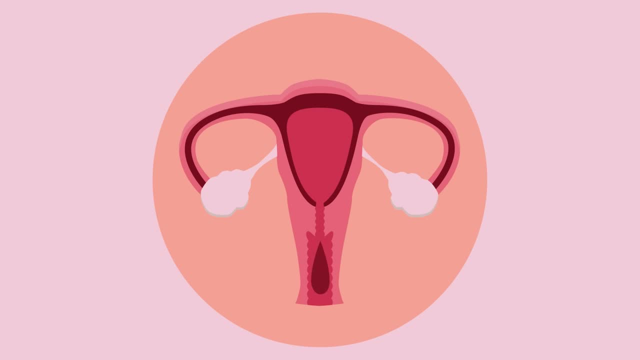 uterus prepares for pregnancy. It prepares for a fertilized egg to settle and grow into a baby. If pregnancy does not occur, the lining breaks down and is expelled from the uterus. This is known as menstruation. The menstrual cycle usually lasts about 28 days During 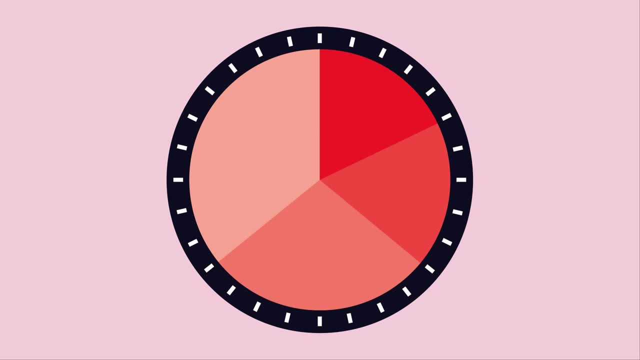 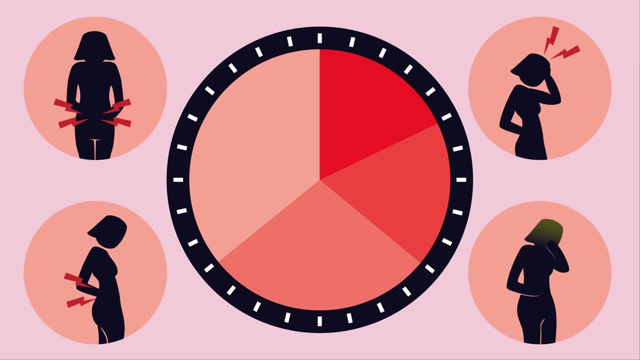 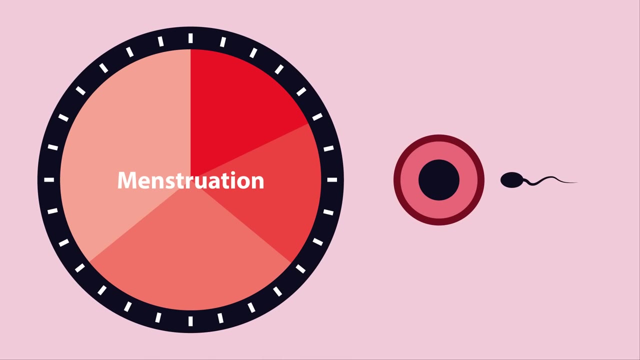 this period, women undergo drastic hormonal fluctuations, as well as physical discomforts such as abdominal cramps, headaches, backaches and general nausea. This has led to it being colloquially referred to as the curse. The first stage of the cycle is menstruation and occurs if the egg has not been fertilized. 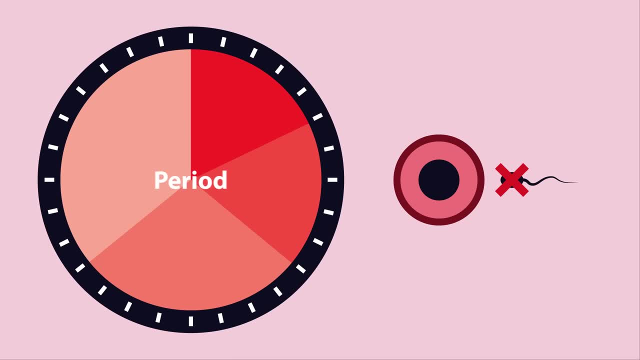 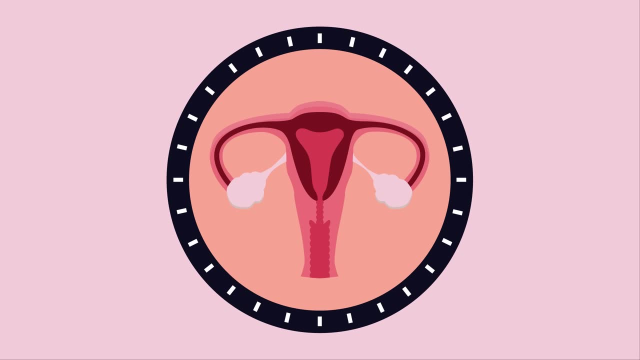 This lasts between three to seven days, and is more commonly known as a period, Because the egg has not been fertilized, the uterus lining, called the endometrium, is not needed, and hence it breaks down and is lost through the vaginal canal with some blood. 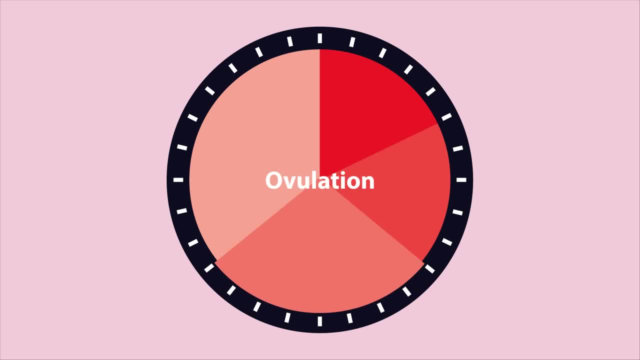 The next stage is known as ovulation and is when the woman is most fertile. After menstruation, the lining of the uterus thickens up again in preparation for a fertilized egg, and inside the ovary a follicle develops. At about 14 days into the cycle an egg is released from. 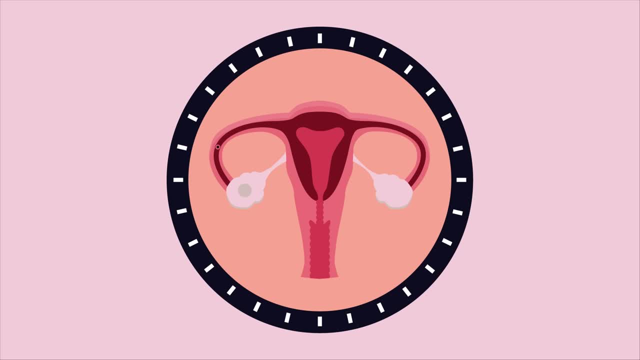 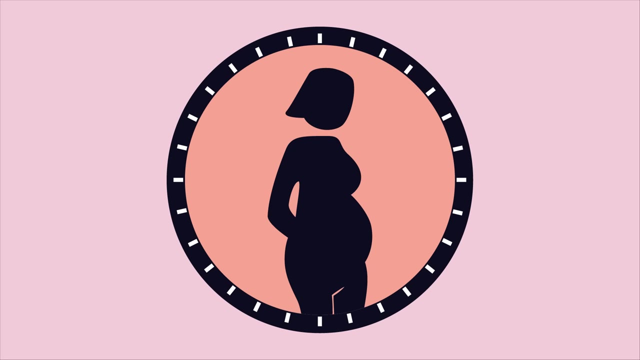 the follicle in the ovaries and fertilization could take place. If the egg is fertilized and embeds itself in the thick uterine lining, the lining is not shed and thus menstruation does not occur and the woman becomes pregnant. If it does not manage to embed, then the lining will break down and menstruation will. 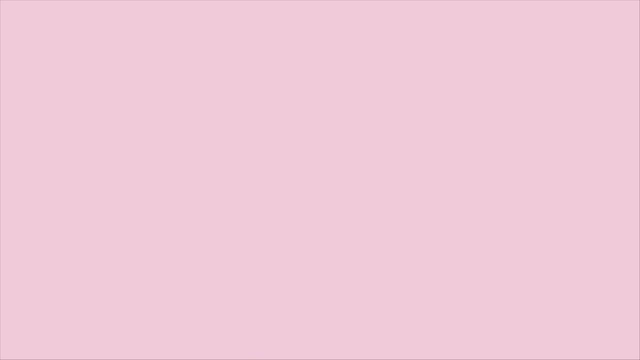 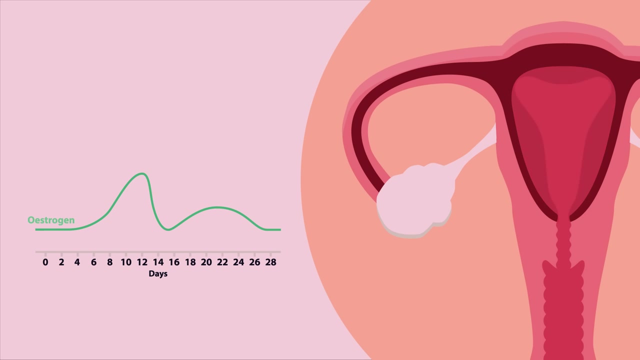 occur and the cycle is repeated. The menstrual cycle is controlled by two main hormones: estrogen and progesterone. We met these hormones in this video. Estrogen is produced by the ovaries and causes the uterus lining the endometrium to thicken.